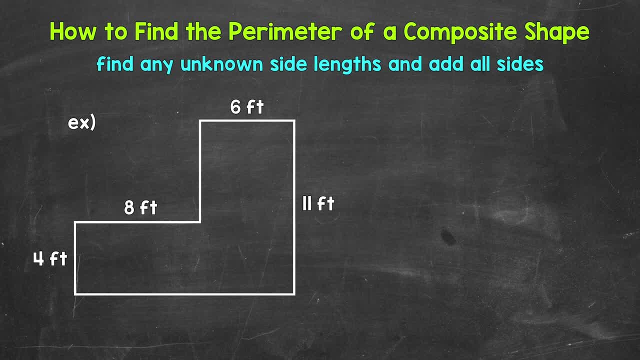 around the outside of a shape. We need to add all of the sides in order to find the perimeter of something. The first thing that we need to do is find any missing side lengths- if there are any, because we will need all of the side lengths in order to find the perimeter For our example. 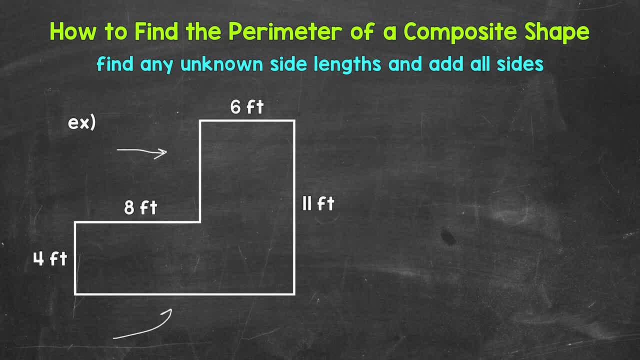 we have two that are missing: This side and this side. We need to use what we know- so what we are given- to figure out what we do not know. For example, we know that this vertical side right here measures the area of a composite shape. We need to add all of the sides in order to find. 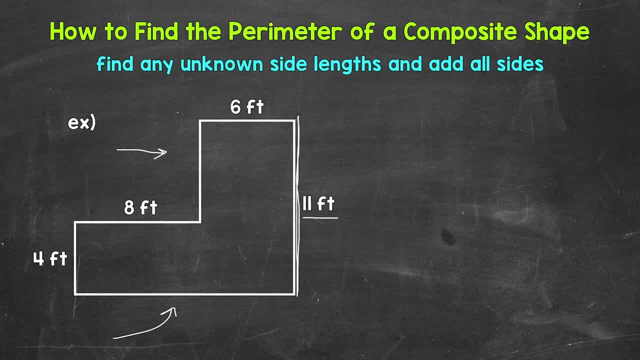 11 feet. We can use that to figure out what this missing side equals. We know that this is 4 feet plus what will give us that 11 feet. Those two vertical sides need to equal 11 feet. Well, 4 feet plus 7 feet equals 11 feet. So that missing side length equals 7 feet. because, again, 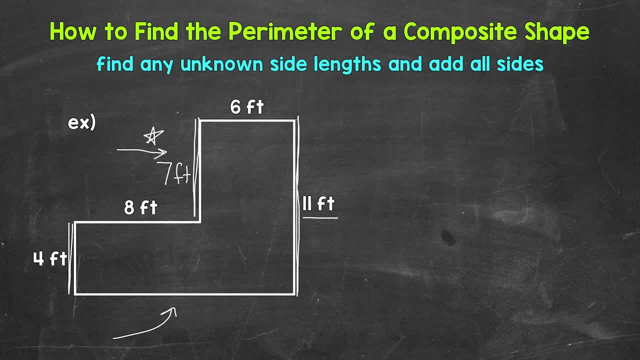 we have 4 feet plus 7 feet. We need to add all of the sides in order to find the perimeter, gives us that 11 feet. Now we can figure out this missing side length right here, So this horizontal side. Again, we need to use what we know, what we are given, to figure out that missing. 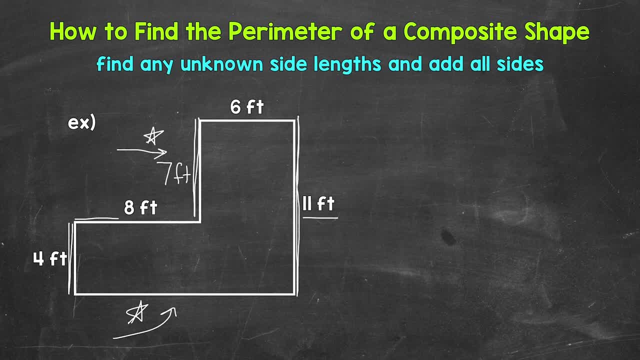 side length. So let's use these two horizontal lines Right here. we have 8 feet and we have 6 feet. Those two sides are going to equal that missing side length. So we have 8 feet plus 6 feet gives us 14 feet. So that missing side length measures 14 feet. Now we can add all of the sides. 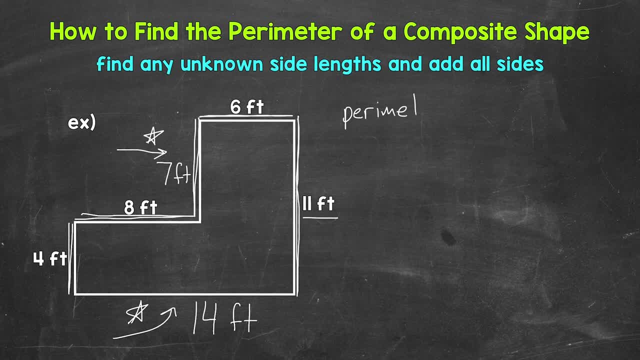 in order to find the perimeter. So perimeter equals- and I will start with 6 feet here- So 6 plus 11.. And I'm going to cross off the sides as I go around, That way I make sure I don't forget anything or count anything twice. So next we have 14 plus 4 plus 8 plus 7.. So 6 plus 11 is 17. 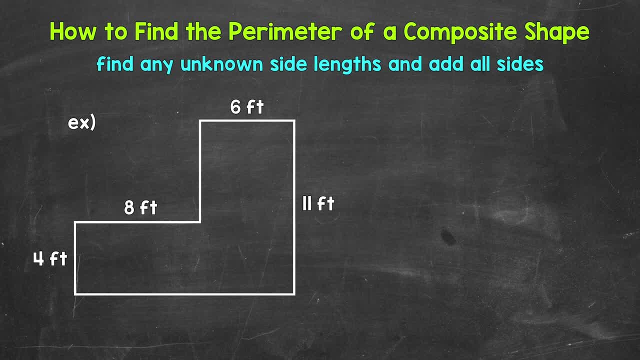 around the outside of a shape. We need to add all of the sides in order to find the perimeter of something. The first thing that we need to do is find any missing side lengths- if there are any, because we will need all of the side lengths in order to find the perimeter For our example. 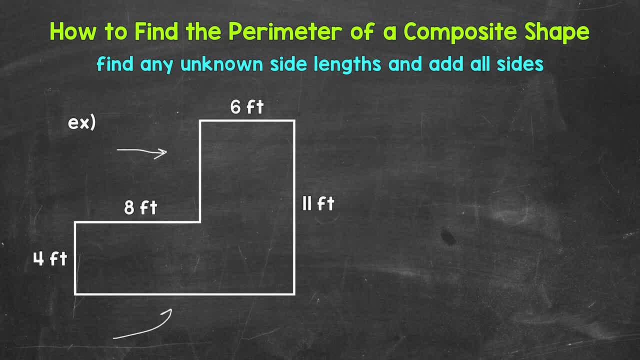 we have two that are missing: This side and this side. We need to use what we know- so what we are given- to figure out what we do not know. For example, we know that this vertical side right here measures the area of a composite shape. We need to add all of the sides in order to find. 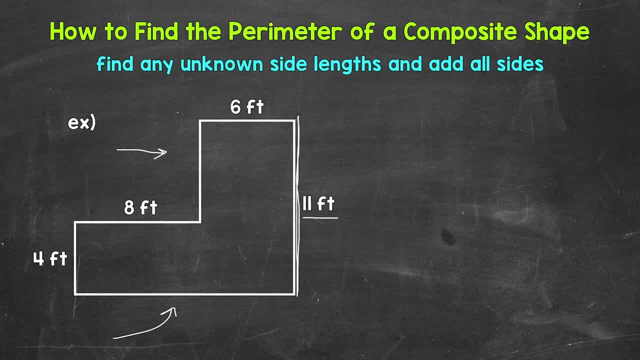 11 feet. We can use that to figure out what this missing side equals. We know that this is 4 feet plus what will give us that 11 feet. Those two vertical sides need to equal 11 feet. Well, 4 feet plus 7 feet equals 11 feet. So that missing side length equals 7 feet. because, again, 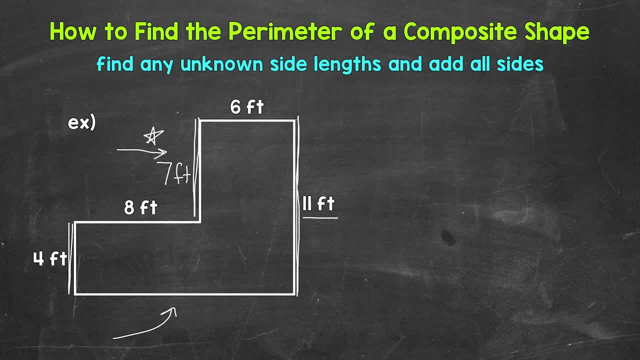 we have 4 feet plus 7 feet. We need to add all of the sides in order to find the perimeter, gives us that 11 feet. Now we can figure out this missing side length right here, So this horizontal side. Again, we need to use what we know, what we are given, to figure out that missing. 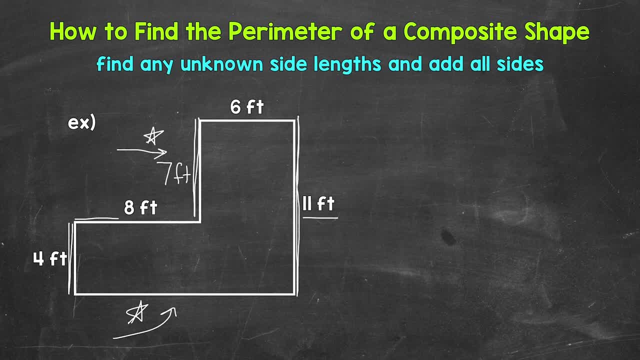 side length. So let's use these two horizontal lines Right here. we have 8 feet and we have 6 feet. Those two sides are going to equal that missing side length. So we have 8 feet plus 6 feet gives us 14 feet. So that missing side length measures 14 feet. Now we can add all of the sides. 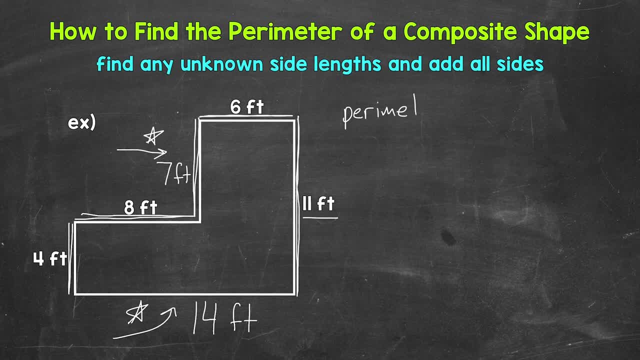 in order to find the perimeter. So perimeter equals- and I will start with 6 feet here- So 6 plus 11.. And I'm going to cross off the sides as I go around, That way I make sure I don't forget anything or count anything twice. So next we have 14 plus 4 plus 8 plus 7.. So 6 plus 11 is 17. 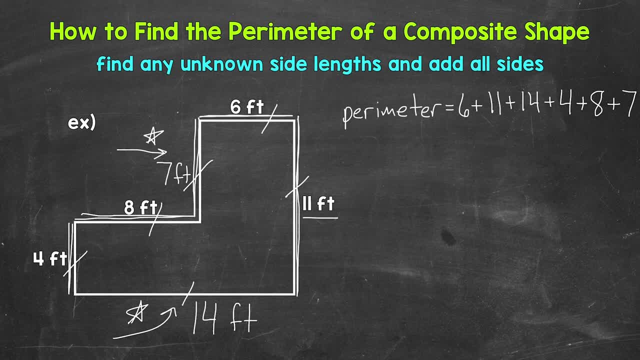 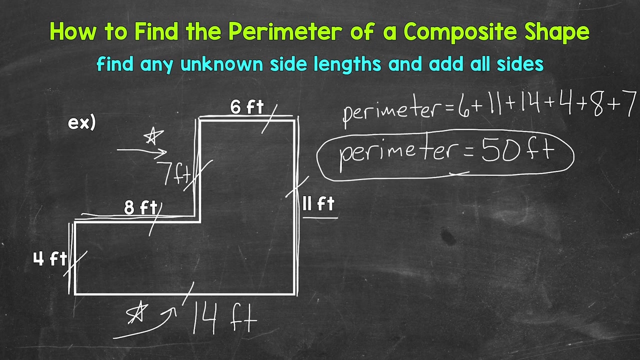 plus 14 is 31, plus 4 is 35, plus 8 is 43.. Plus 7 is 50. So the perimeter equals 50 feet. So that's how we find the perimeter. Let's move on to finding the area. Now remember, area is the. 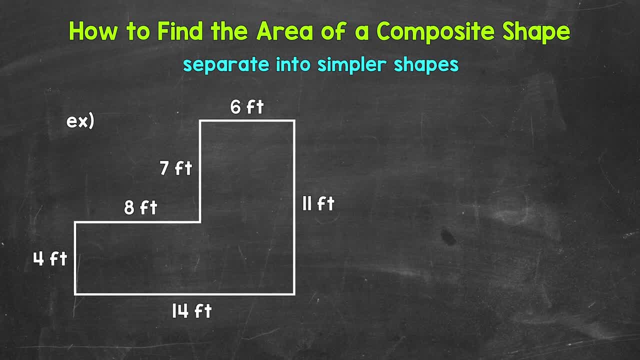 amount of space or surface inside of a shape. So how much space or surface something covers. When we find the area of the perimeter, we find the area of the perimeter. So we find the area of the composite shapes. We can separate the shape into simpler shapes. We find the area of those shapes. 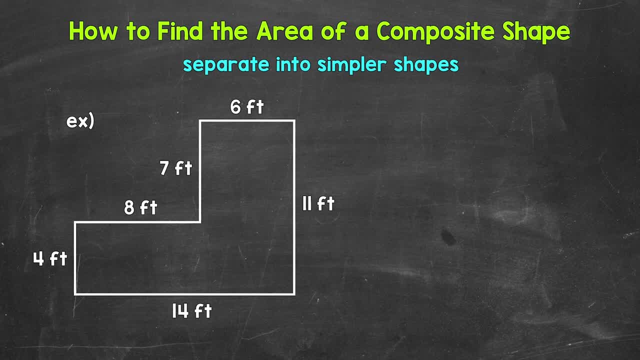 and then add them together to find the total area. Let's jump into our example And you'll notice we don't have a simple rectangle, square, triangle or whatever the case may be that we can easily find the area of. So let's separate this shape or break this figure up into simpler shapes. So let's. 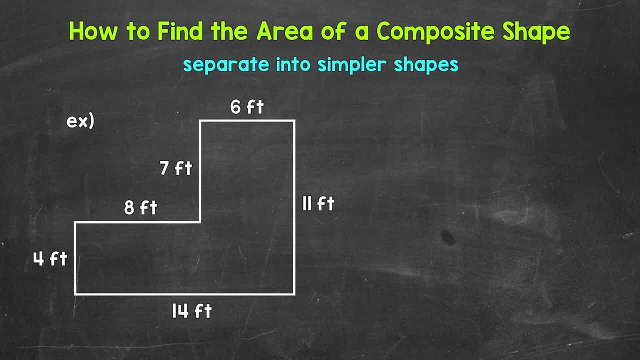 create a new rectangle, and we'll finish this scene here. So let's do that. Let's create another. Let's start by finding the area of view from the bottom rectangle, finding the area of A, and, since it is a rectangle, let's use the formula area. 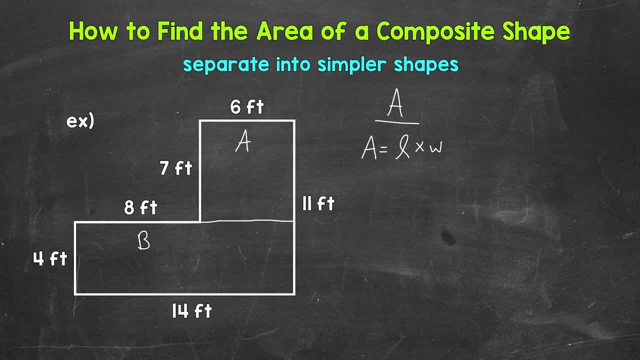 equals length times width. Now I'm using a cursive L. that way it doesn't look like a 1.. Now we need to find the correct length and width for rectangle A. Well, this is a 7 by 6 rectangle, so let's plug those in 7 times 6.. It's very important. 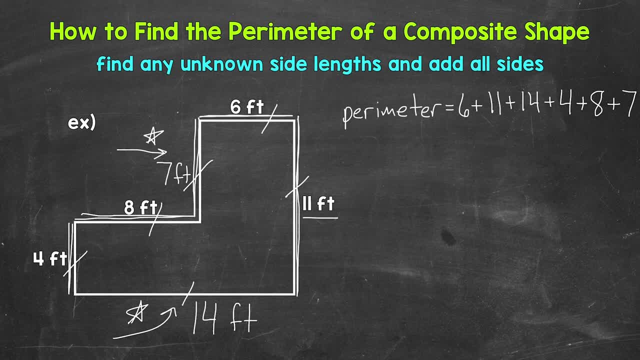 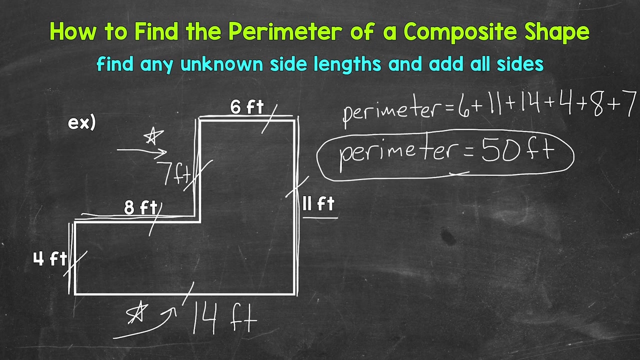 plus 14 is 31, plus 4 is 35, plus 8 is 43.. Plus 7 is 50. So the perimeter equals 50 feet. So that's how we find the perimeter. Let's move on to finding the area. Now remember, area is the. 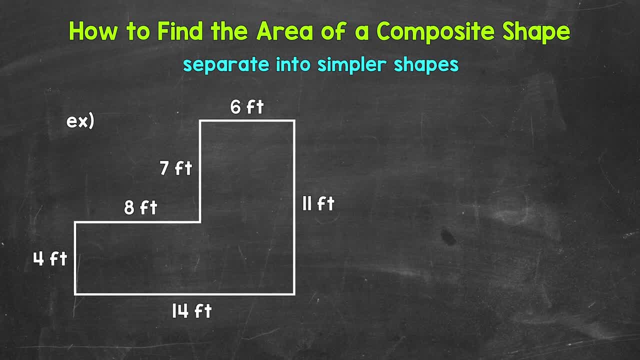 amount of space or surface inside of a shape. So how much space or surface something covers. When we find the area of the perimeter, we find the area of the perimeter. So we find the area of the composite shapes. We can separate the shape into simpler shapes. We find the area of those shapes. 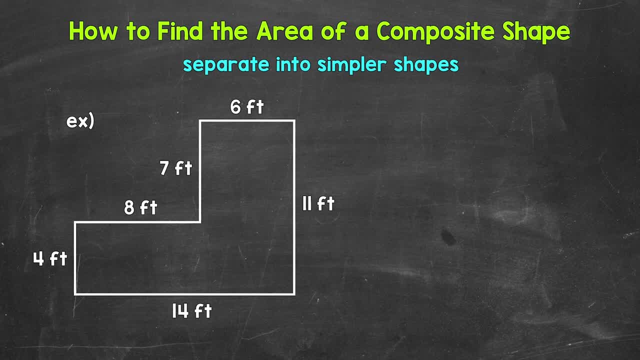 and then add them together to find the total area. Let's jump into our example And you'll notice we don't have a simple rectangle, square, triangle or whatever the case may be that we can easily find the area of. So let's separate this shape or break this figure up into simpler shapes. So let's. 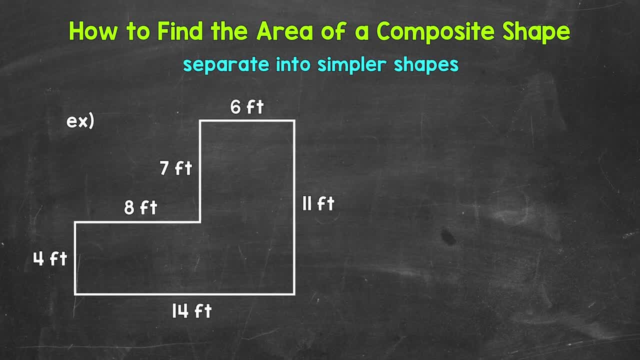 start doing the same. So let's find the area of the perimeter. So there's this particular piece called a square here, And since I've paste this in 4 data facts group that you're going to get this table, So let's sociedade this as a square up here. So what we're going to do is read this: 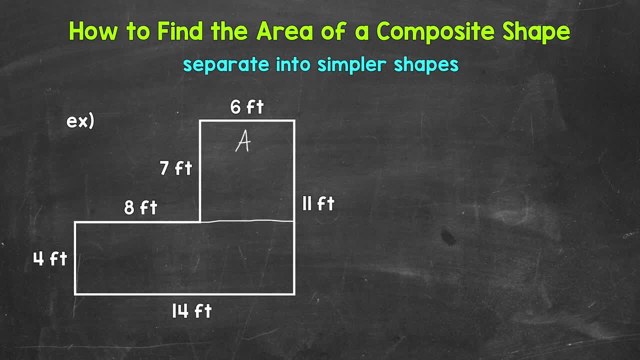 in our image. This is just a사� означ module And we need to create a section. So when we do that, isanna is sufficient and triangle does not, finding the area of A, and since it is a rectangle, let's use the formula area. 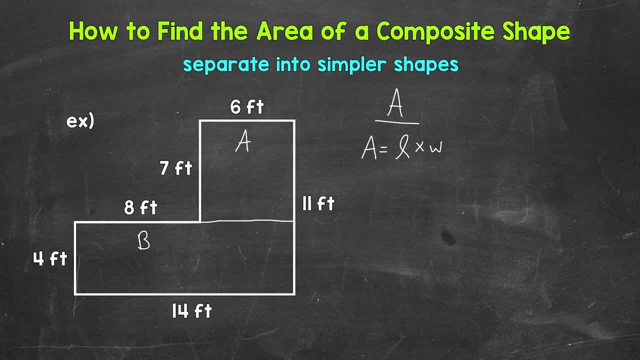 equals length times width. Now I'm using a cursive L. that way it doesn't look like a 1.. Now we need to find the correct length and width for rectangle A. Well, this is a 7 by 6 rectangle, So let's plug those in 7 times 6.. It's very important. 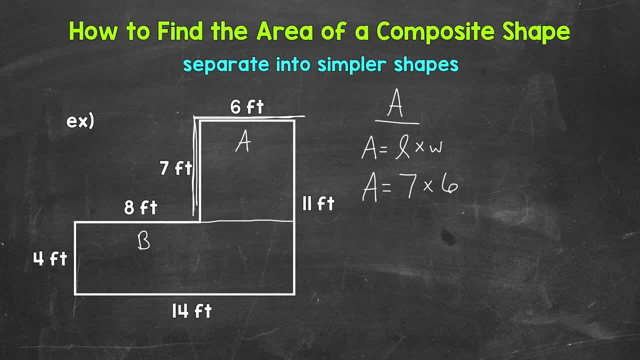 that we pick the correct length and width for the given rectangle, For example. we don't need this 11 feet here. that goes all the way down here. So be careful about which side lengths you are using for can calculating the area I also want to mention. don't get too held up on which is the length and which. 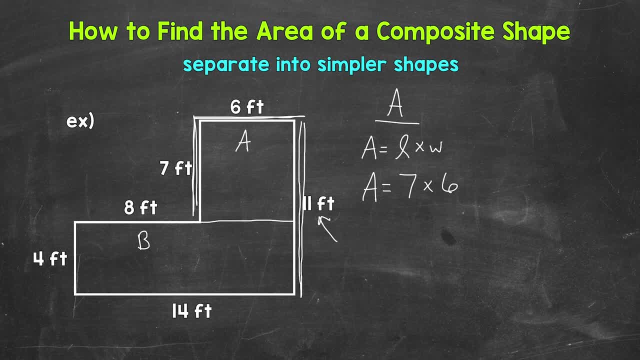 is the width. I'm using the longer side length for the length to keep it consistent, but really you're going to get the same area either way. So, in my opinion, don't get too held up on which is the length and which is the width. Just make sure you are using the correct sides for calculating. 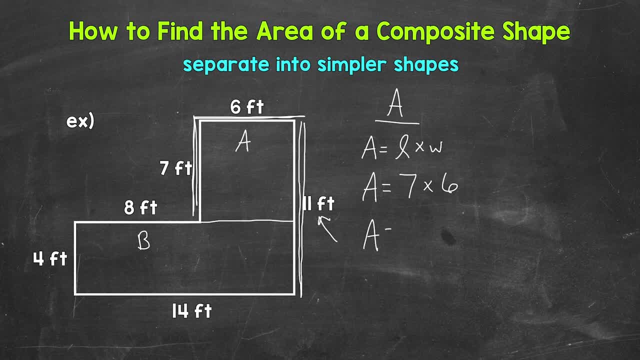 that area. So as far as the area for A, 7 times 6 gives us 42, and this is square feet, So the area here is 42 square feet. Now we need to find the area of B, So area equals length times width. 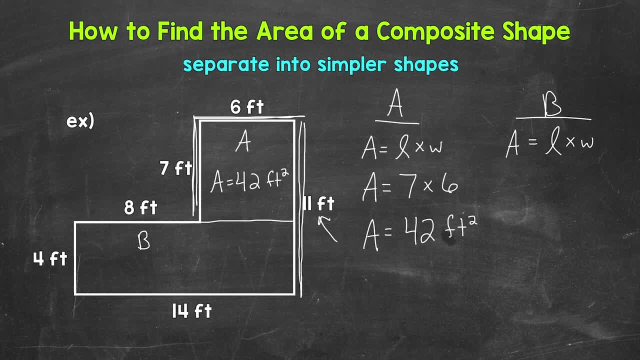 So now let's pick out the correct sides Here. as far as what we need to calculate the area, This is a 14 by 4 rectangle, So 14 feet by 4 feet, So let's plug those in Again. I'm using the 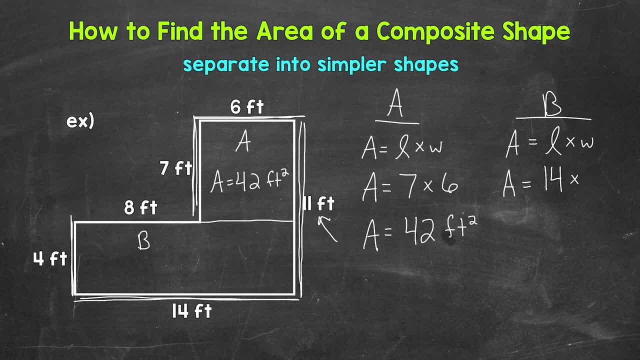 longer side length for the length, So 14 times 4.. Now, before we multiply 14 times 4, I do want to mention we did not need this 8 feet because that's the length that we're going to be using for the area. So we're going to need: 14 times 4.. Now, before we multiply 14 times 4, I do want to mention we did not need this 8 feet because that's the length that we're going to be using for the area. So that's the length that we're going to be using for the area. 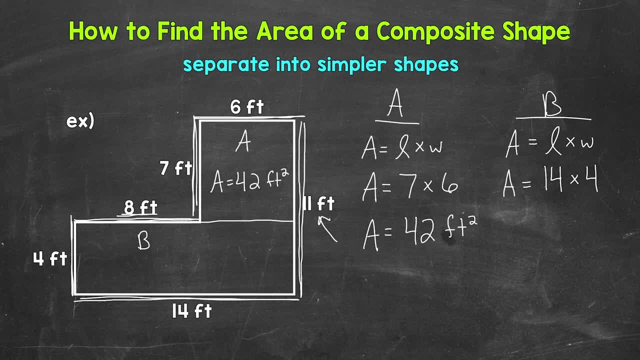 That only goes to that point. We needed the 14 feet all the way across the bottom of that rectangle. So again, we need to be careful as far as which side lengths we are using. So now, let's multiply 14 times 4 equals 56. So the area of B is 56 square feet. 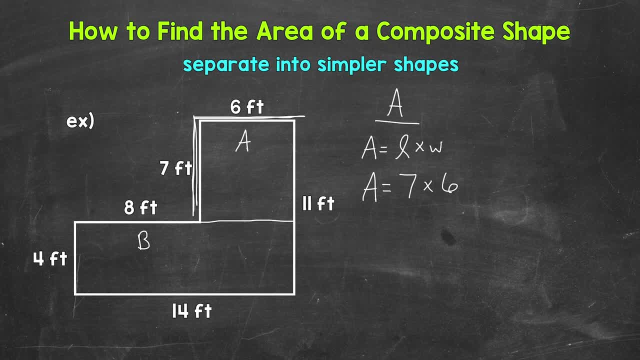 that we pick the correct length and width for the given rectangle. For example, we don't need this 11 feet here. that goes all the way down here. so be careful about which side lengths you are using for rectangle A. I also want to mention: don't get too held up on which is the length and which. 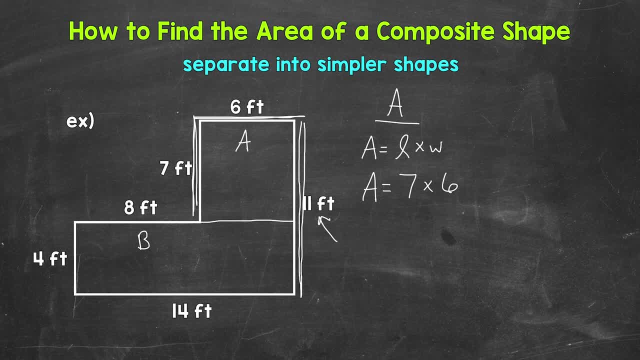 is the width. I'm using the longer side length for the length to keep it consistent, but really you're going to get the same area either way. so in my opinion, don't get too held up on which is the length and which is the width, Just. 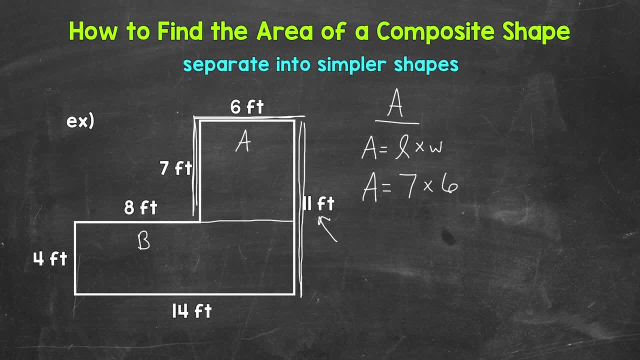 make sure you are using the correct sides for calculating that area. So, as far as the area for the rectangle A is the length and which is the width, Don't get too held up on which is the length and than decide where the length and the width are. 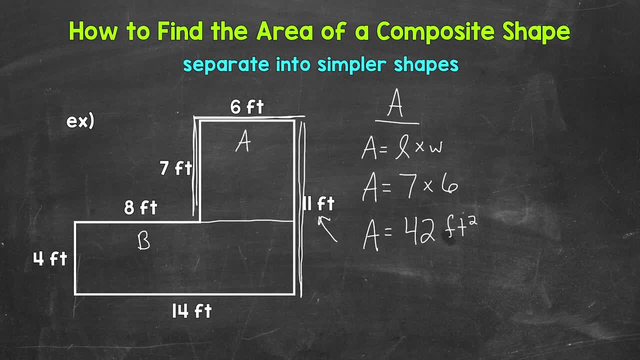 For example, the area for article A is 45 by 22 and the height is 42 and this is the length on both the sides. so we a need an area for article A.7767 times 6 gives us 42 and this is square feet. so the area here is 42 square feet. Now we need to find the area of B, So area equals length times width. So now we have to pick out the correct sides here as far as What we need to calculate: the area Number- that means X- and the length, If there's one number equal to counter plus the Rick. 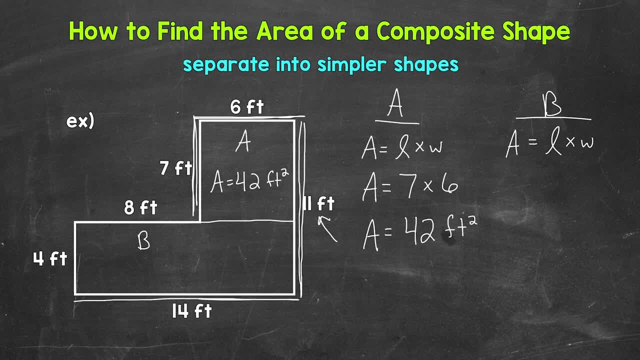 this is a 14 by 4 rectangle, so 14 feet by 4 feet, so let's plug those in again. I'm using the longer side length for the length, so 14 times 4. now, before we multiply 14 times 4, I do want to mention 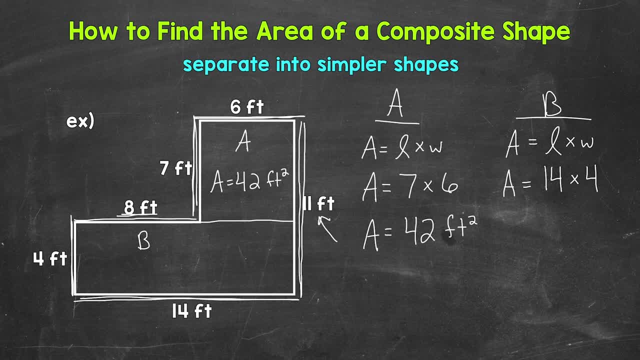 we did not need this 8 feet, because that only goes to that point. we needed the 14 feet all the way across the bottom of that rectangle. so again, we need to be careful as far as which side lengths we are using. so now let's multiply 14 times 4 equals 56, so the area of b is 56 square feet.